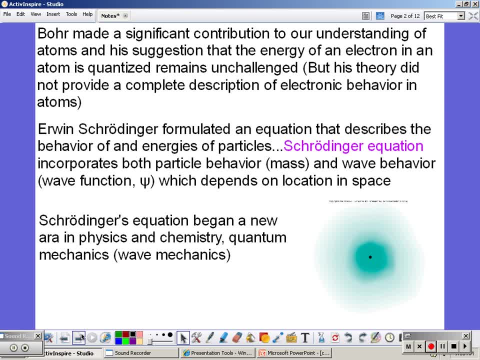 energy of an electron in an atom is quantized remains unchallenged. But his theory did not provide a complete description for electronic behavior in atoms. Erwin Schrödinger formulated an equation that describes the behavior and energies of particles, So Schrödinger's equation incorporates both the particle behavior, the 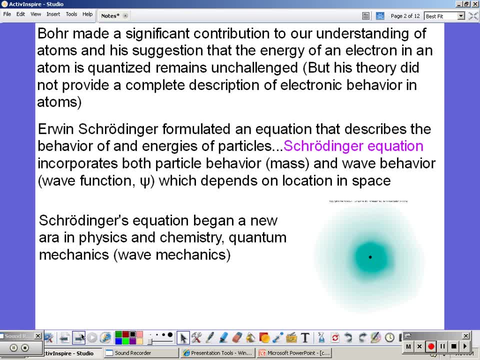 mass and wave behavior, which is the way function, which depends on the in space or the location of the electron in the atom. So Schrodinger's equation began a new era in physics and chemistry called quantum mechanics or wave mechanics. Now his equation is high calculus, which is beyond the scope of this class. but if we 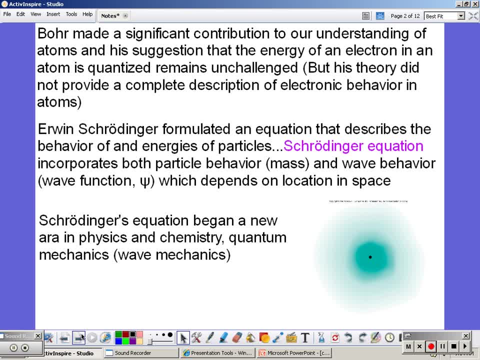 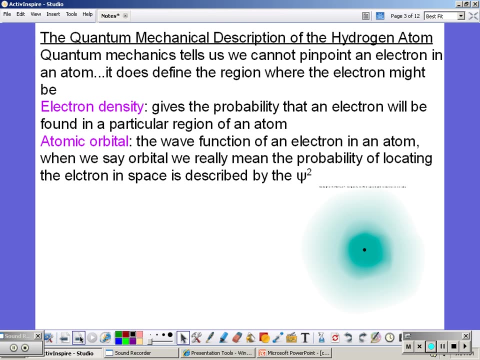 calculated where the electron most probably is located, then we get these pictures called electron densities. So if we plot where the electron should probably be located, we actually start seeing a shape of these electron clouds. So the quantum mechanical description of the hydrogen atom tells us we cannot pinpoint. 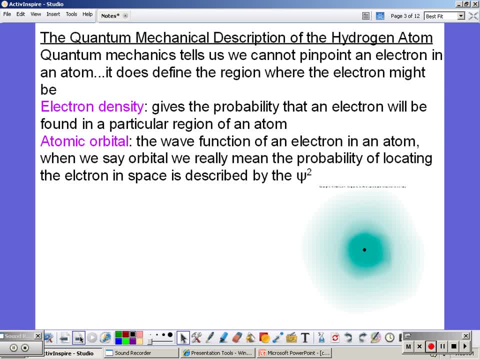 an electron in an atom, but it does define the region or these 3D areas. this electron density picture where the electron might be. So electron density gives us the probability of the electron Where it should be found. The atomic orbital is the wave function of the electron in the atom. 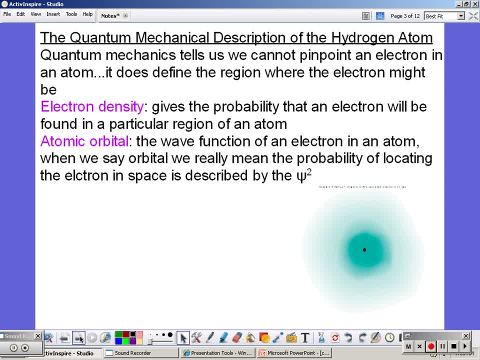 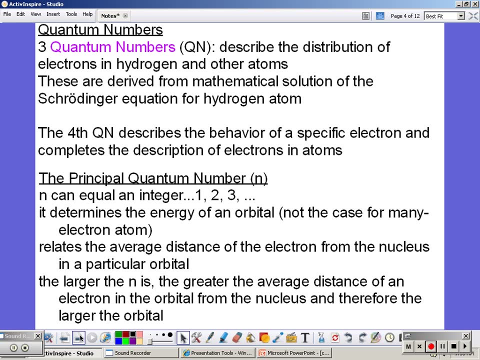 So when we say orbital, we're really meaning the probable location of the electron in space described by the wave function squared. And that wave function, remember, is coming from Schrodinger's wave equation. Quantum numbers are used to describe the distribution of electrons in the hydrogen atom and others. 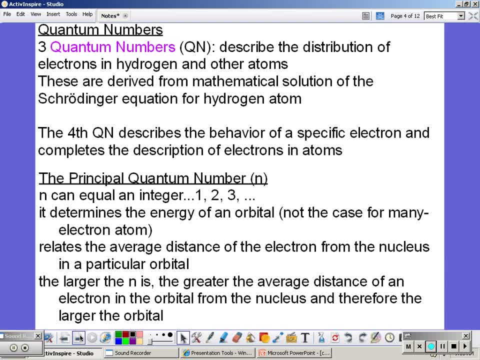 These are derived mathematically from the Schrodinger equation. Now the fourth quantum number describes the behavior of this specific electron and completes the description of the electrons in the atoms. So the first three numbers all come from Schrodinger's wave equation, and the fourth one describes 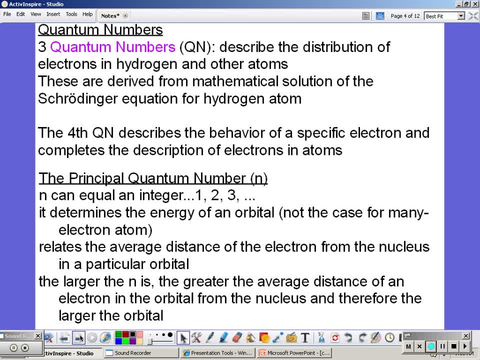 that specific electron. So the first quantum number is the principal quantum number, or n. N can equal an integer, so it has to be 1,, 2,, 3,, 4,, 5, 6,, so on and so forth. 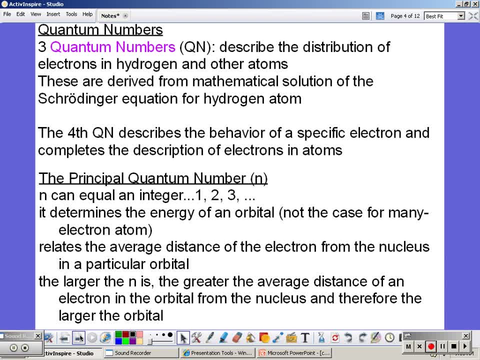 It determines the energy of the orbital, Although not the case for many electron atoms and we'll get to that later. It relates the average distance of the electron from the nucleus in a particular orbital. The larger the n value is, the greater the average distance from the electron is from. 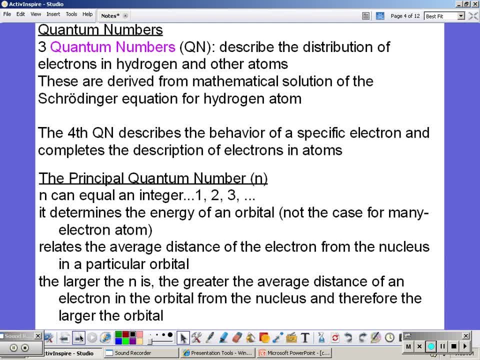 the nucleus and therefore the larger the orbital. So when we're on the first energy level, n is equal to 1, and we're close to the nucleus, N is equal to 2.. We're a little bit farther out, and so the orbital gets larger. 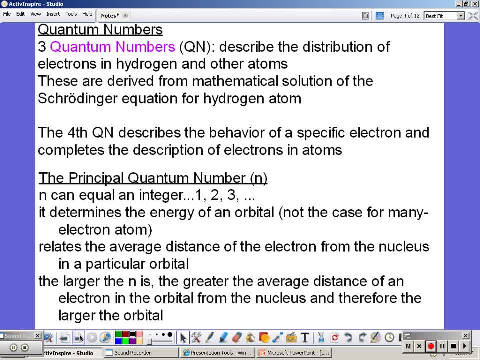 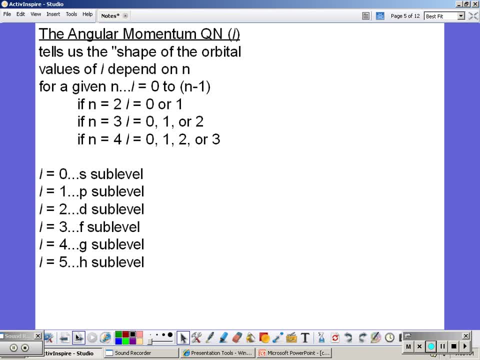 N is equal to 3.. We're on the third energy level, the third principal quantum number, and it's an even larger orbital. The angular momentum quantum number, or L, tells us the shape of the orbital, and its values depend on n. 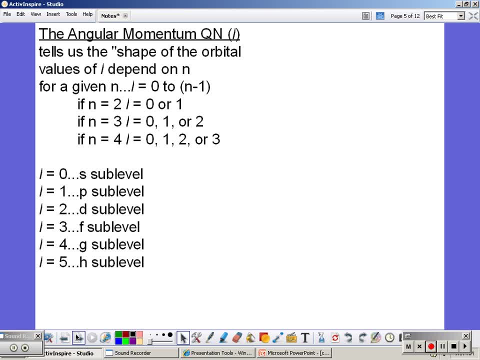 So for a given n, let's say n is equal to 1,, then L has to be equal to 1.. If n is equal to 0,, all the way up to n is equal to 1.. So if n is equal to 1, L has to equal 0.. 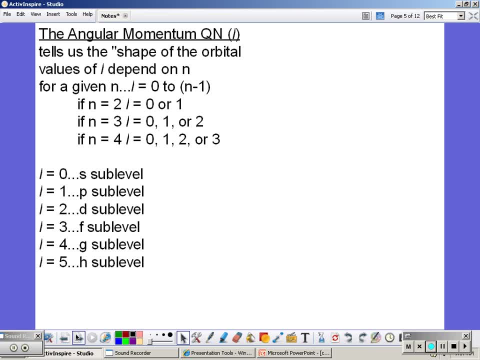 If n is equal to 2, L has to equal 0 or 1.. If n is equal to 3,, then L has to equal 0,, 1, or 2.. If n is equal to 4,, you have 0,, 1,, 2, or 3, and so on and so forth. 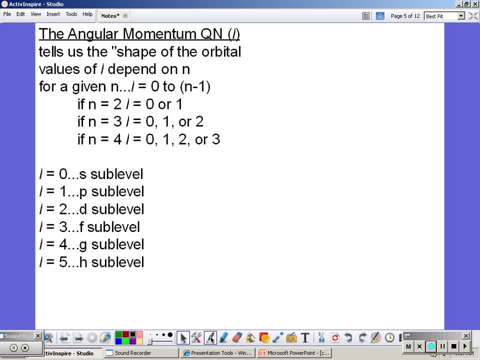 So what those L values are telling us are our sublevels. So the 0 represents our s. So if we look at, n is equal to 2, then we can have a 2s. or 1 is p, so we could have a 2p. 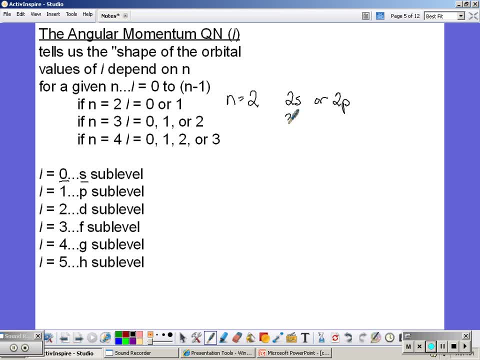 3, we have a 3s or a 3p or a 3d, So the angular momentum quantum number is telling us the sublevel which we label spd or f, and you can theoretically keep going. So after you get to f, you just start going. 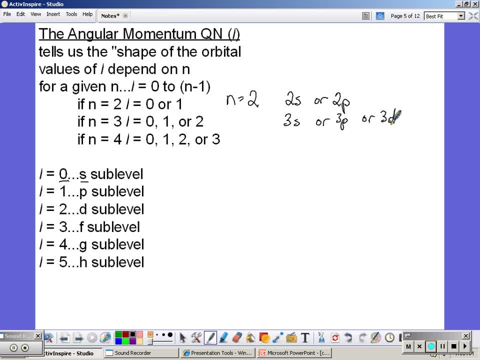 So you can theoretically keep going. So you can theoretically keep going based on the alphabet f, g, h, i and you would skip over s and p. The third quantum number is the magnetic quantum number, m sub L. It describes the orientation. 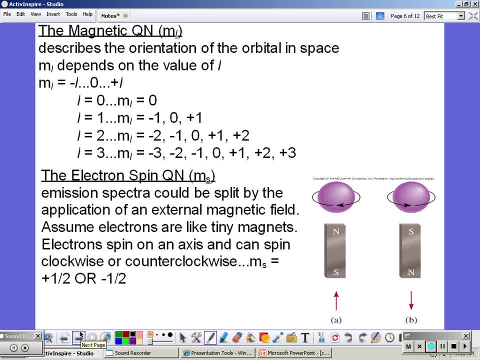 of the orbitals in space. M sub L depends on the value of L. So the m sub L value would go from a negative L through 0 up to the positive L. So if L is equal to 0. M sub L has to equal 0.. 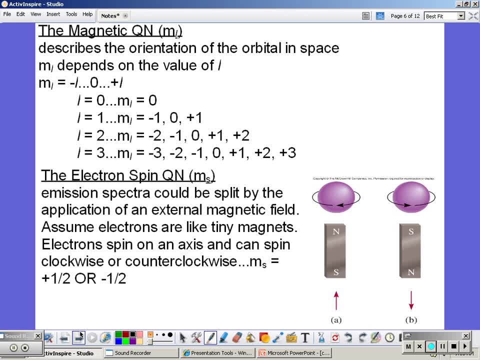 If L equals 1, m sub L has to equal negative 1, or 0, or plus 1.. If L is equal to 2,, then m sub L has to equal negative 2,, negative 1, or 0, or plus 1, or. 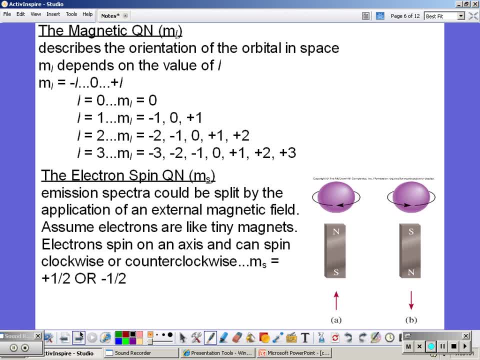 plus 2.. So on and so forth. So remember, these are my sublevels: s, p, d and f. So what the m sub L is describing is the orientation of the orbital in space. So what the m sub L is describing is the orientation of the orbital in space. 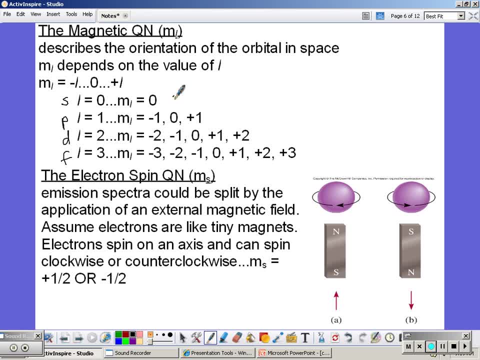 So what the m sub L is describing is the orientation of the orbital in space. So this is my sublevel, This would be my orbital. So the s sublevel has one orbital, The p sublevel has three possible orbitals, The d has four- I'm sorry, five- possible sublevels and the f has seven possible sublevels. 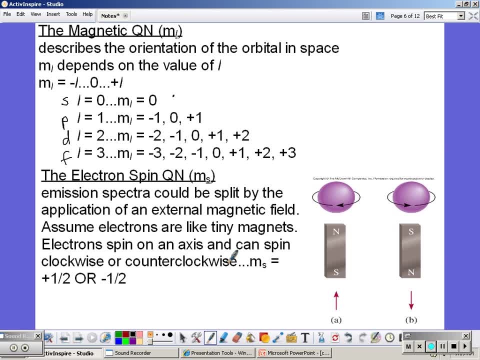 Now the fourth quantum number that's not related to Schrodinger's wave equation is the electron spin. The emission spectrum could be split by the application of the magnetic field. So when we look at the magnetic field we can see that the emission spectrum could be split by the application of the magnetic field. 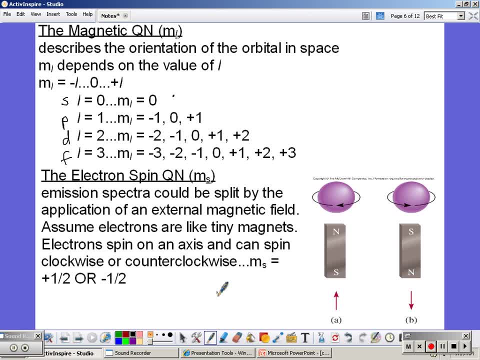 So when we look at the magnetic field, we can see that the emission spectrum could be split by the application of the magnetic field. So when we looked at hydrogen's emission spectrum and we apply a magnetic field, we actually see divisions in the lines or it's split in half. 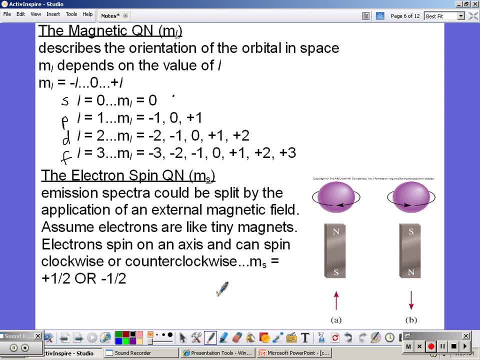 And that's because the electron is spinning. So assume electrons are like tiny magnets. The electrons spin on an axis and can spin clockwise or counterclockwise. So m sub s either is a plus one half or a minus one half, And it doesn't matter which value we apply, but it has to be plus one half. 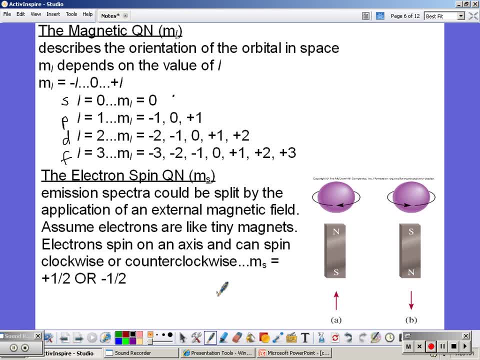 And it doesn't matter which value we apply, but it has to be plus one half or a minus one half. When we draw our orbital notations, we show that using the up and down arrow. Alright, so this is just a table of our quantum numbers that are based on Schrodinger's. so 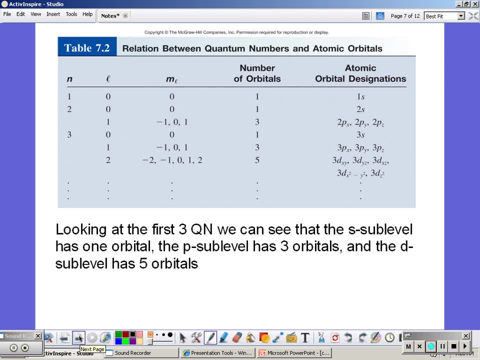 just the first three. So looking at the first two quantum numbers, we can see that the? s sublevel has one orbital, one s The p sublevel has three orbitals, and the first time it shows up is in our second energy level. 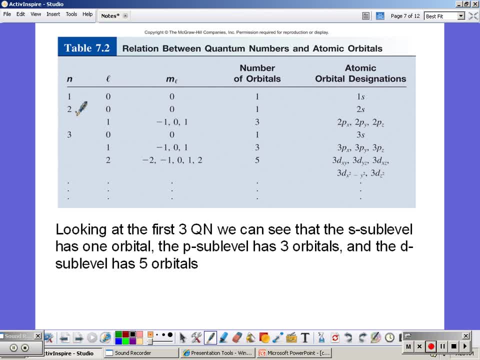 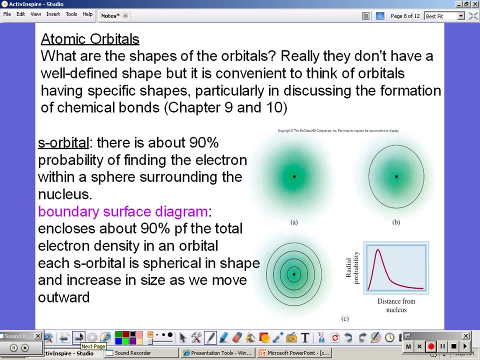 The third or the d sublevel has five orbitals and it first shows up in our 3d or in our third energy level, So atomic orbitals. What are the shapes of these orbitals? They really don't have a well-defined shape, but it's convenient to think about the orbitals. 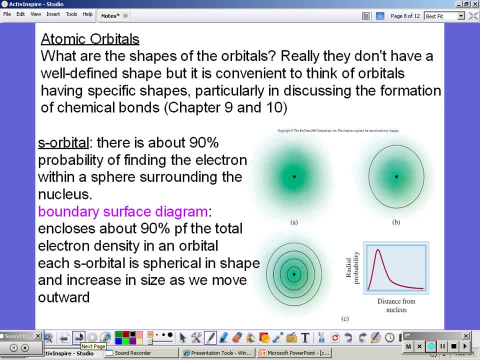 having specific shapes, particularly when we start discussing information of chemical bonds in chapters nine and ten. So the s orbital. There is about a ninety percent probability of finding the electron within a sphere surrounding the nucleus. So if you look at your electron densities you can see that when we plot those diagrams, 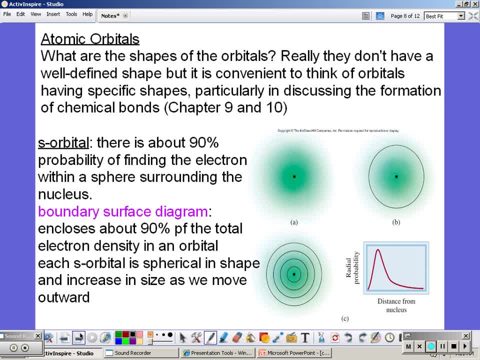 they tend to look like a sphere If we keep coming out from the nucleus, if we start to calculate those values of the different energy levels, they still look like a sphere. but the sphere is getting larger and larger. So the boundary surface diagram encloses about ninety percent of the total electron density. 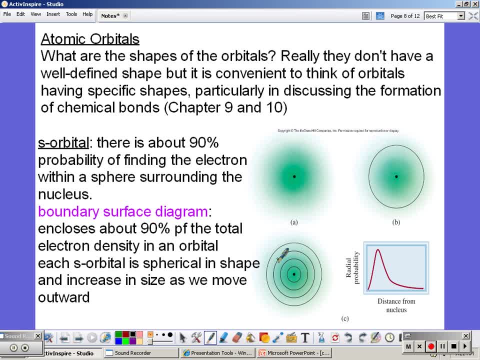 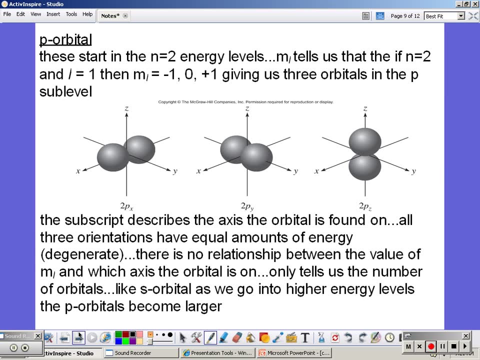 in an orbital. Each s orbital is spherical in shape and increases its size as we move outward. As we increase the size, as we move outward, we're also increasing the amount of energy. Now the p orbital. These start again in the second energy level, and m sublevel tells us that if n is equal, 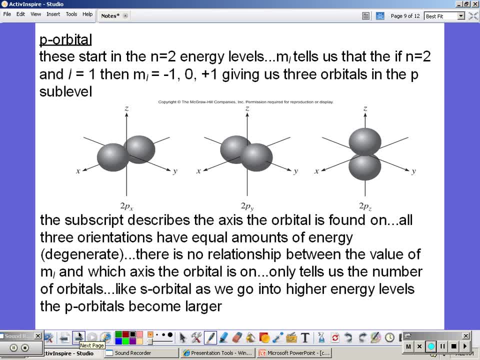 to two and l is equal to one, then m sublevel has to be negative, one, zero or plus one. So we get three different views. So if we look at the diagram, this subscript here- x, y and z- describes the axis that 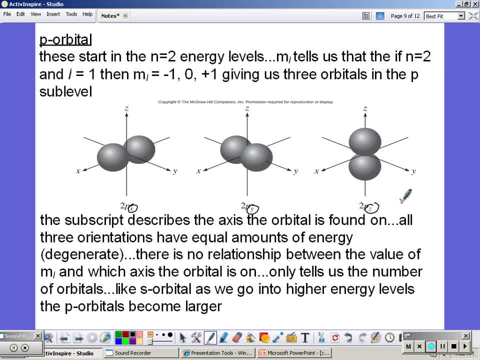 the orbital is found on. All three orientations have the equal amount of energy, so there's really no difference between 2px, 2py and 2pz, So they're degenerate. There's also no relation to the m sublevel values: negative one, zero or plus one. 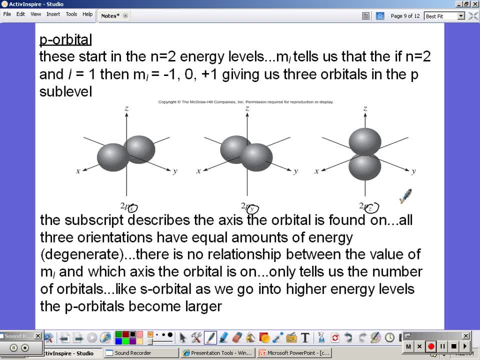 All the m sublevel is telling us is that there are three possible orientations. When we graph those orientations, that's where we get the subscript from. Like the s orbital, as we go into higher energy levels the p orbitals become larger. 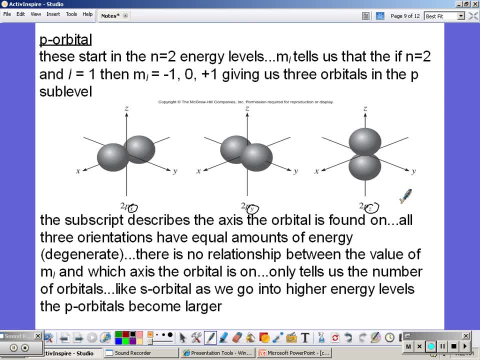 So you have your 2p. Your 3p would be larger than your 2p. The 3p would have more energy than your 2p. D orbitals- D orbitals. Now d orbitals- D orbitals. 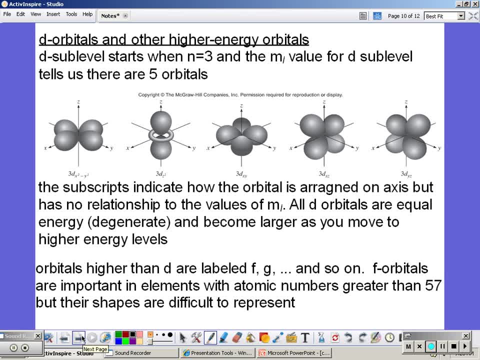 D orbitals. The D sub level starts when N is equal to 3, and so your M sub L value, your L value, would have to be 2.. So your M sub L value would either have to be minus 2, minus 1,, 0, plus 1 or plus 2.. If we were to graph those different areas using the electron densities, 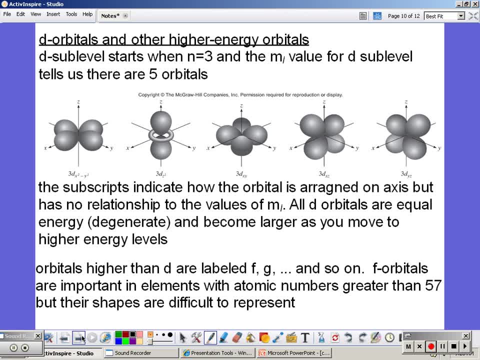 and Schrodinger's wave equation. this would be. these would be what our orbitals would look like. So again, look at your subscripts. They're telling you how the orbitals are in lined with the axis. They don't match up to a negative 2, negative 1, 0, plus 1 or plus. 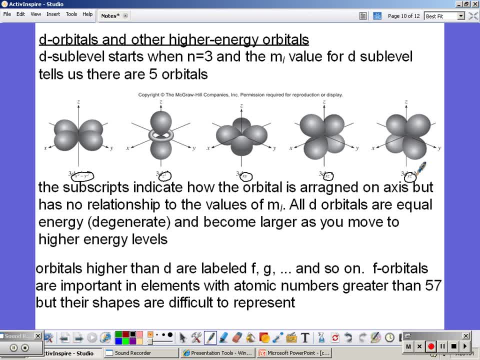 2. It just describes it how it looks on the axis. Remember, your M sub L value is just telling you how many different versions you have. Now all the D orbitals are equal in energy, so they're all degenerate and become larger as you go to higher energy. 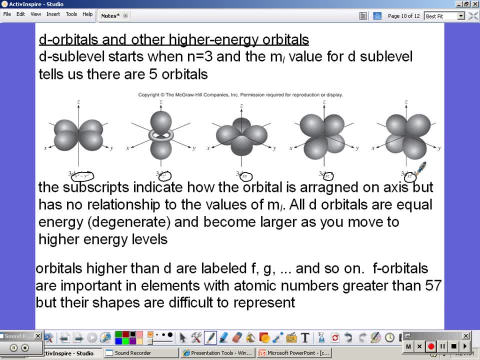 Subtitles by the Amaraorg community. So your 4D is larger than your 3D and your 4D has more energy than your 3D- Any orbitals that are higher than D, like your F specifically. your F is important to atomic numbers greater. 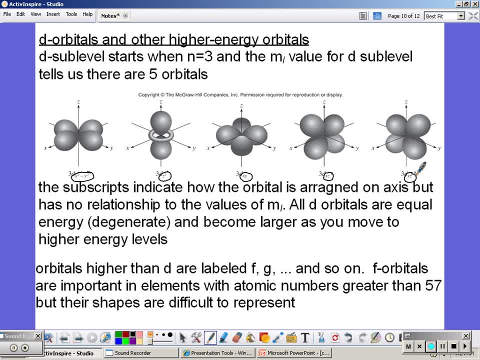 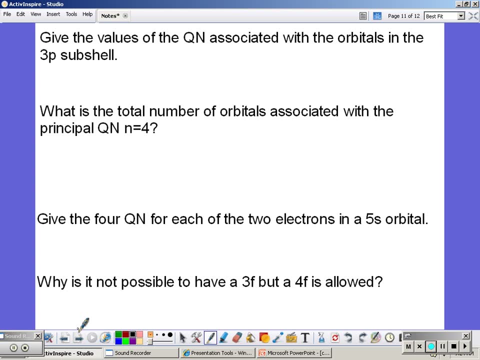 than 57, but their shapes are more difficult to represent. So we're not going to really go past the F orbitals in this level course. Alright, so let's start putting these quantum numbers together. So, given the values of the quantum numbers associated with the orbitals, 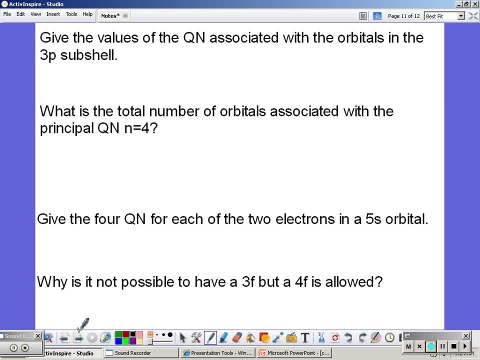 in the 3P sublevel. So the big number there would be our principal energy level, N. So N would have to equal 3.. Well, if N is equal to 3, then L can be 0,, 1 or 2.. Now the P tells: 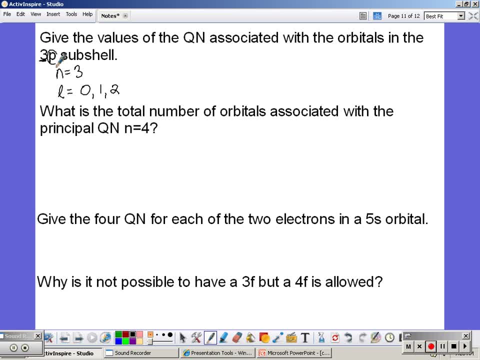 me I'm talking about L is equal to 1.. So if N is equal to 1,, then L is equal to 2.. So if N is equal to 3 and L is equal to 1,, then my M sublevel is going to be negative 1 or. 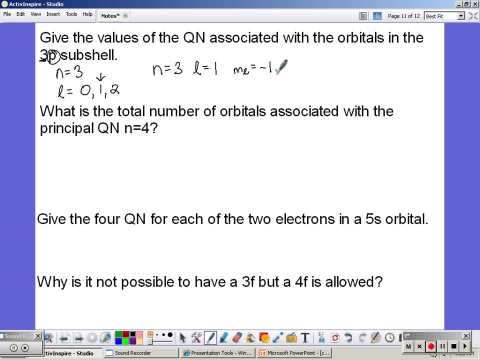 0 or plus 1.. Now, we don't usually write it out like that. We usually just write 3, 1, negative 1.. Or it could be 3, 1, 0. Or it could be 3, 1, plus 1.. So that would be the. 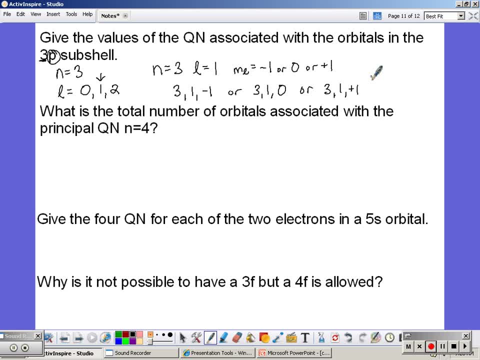 answer to that question: What is the total number of orbitals associated with the principal quantum number? N is equal to 4?. Well, if N is equal to 4, then L is going to be 0,, 1,, 2 or 3.. It goes from 0 up. 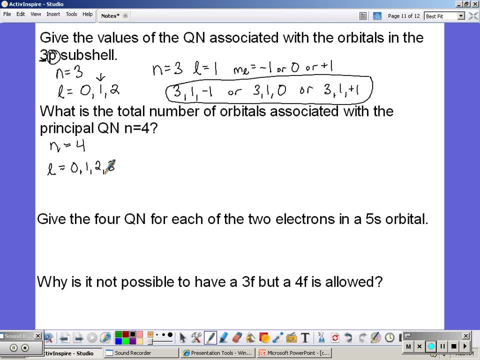 to N minus 1.. Well, if L is equal to 0,, then M sublevel has to equal 0.. If L is equal to 1, then M sublevel equals negative 1.. 0 or plus 1.. If L is equal to 2, M sublevel equals negative 2, negative 1,, 0, plus 1 or. 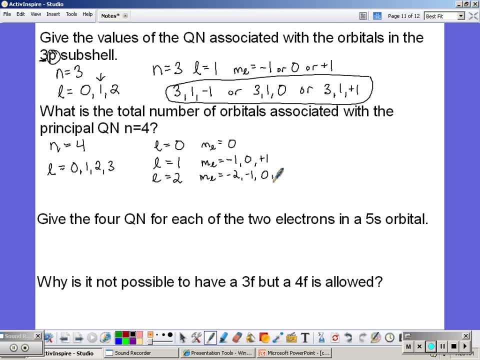 plus 2.. If L is equal to 3, M sublevel equals negative 3, negative 1,, I'm sorry, negative 2, negative 1, 0, plus 1, plus 2 or plus 3.. So how many orbitals do I have? total One. 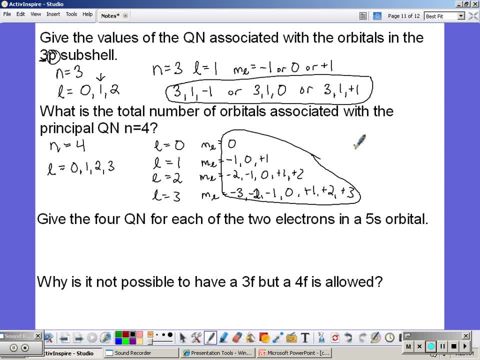 plus 3, plus 5, plus 7.. So that would give me 16 orbitals. Well, if you look at, your N is equal to 4, and we have 16 orbitals. To figure out your number of orbitals then, 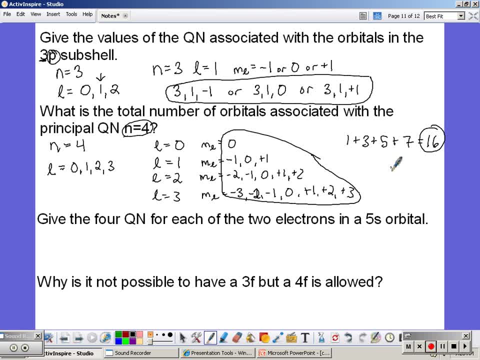 you can simply do N squared. Give the 4 quantum numbers for each of the 2 electrons found in the 5s orbital 5s. So N has to equal 5. 5s, 5s, 5s. 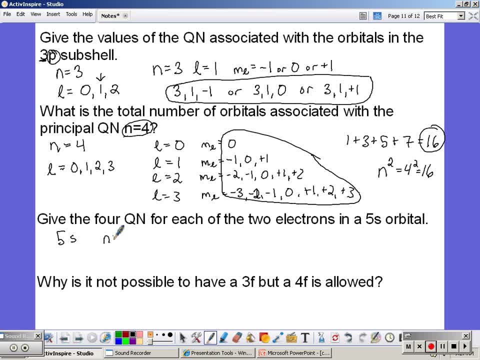 5s, Because I'm in the s sublevel, L has to equal 0.. Because L equals 0, M sublevel also has to equal 0.. Now I want to give it for each of the 2 electrons, So my spin is going to. 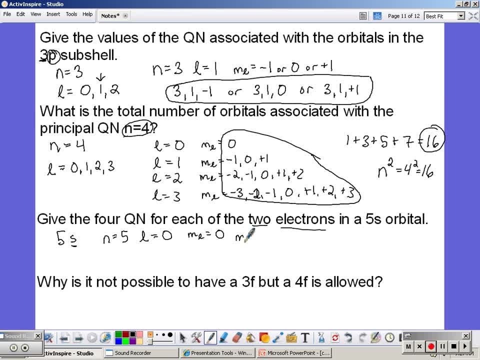 be plus 1 half for one of my electrons. For my other electron it's going to have the same first 3 quantum numbers because it's in the 5s. So the only difference then is going to be that 4th quantum number, and it's going to spin in the opposite direction. 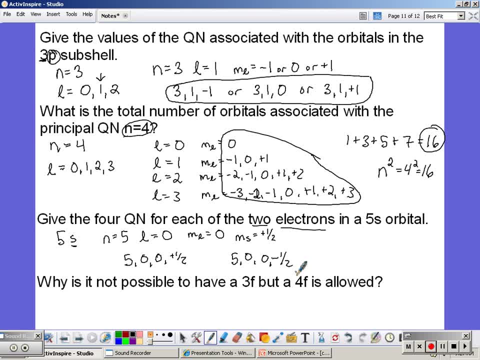 So negative 1 half. Why is it not possible to have a 3f, but 4f is allowed Again, our quantum numbers tell us this. So if N is equal to 3,, then L has to be 0,, 1, or 2.. So f is not a possibility. 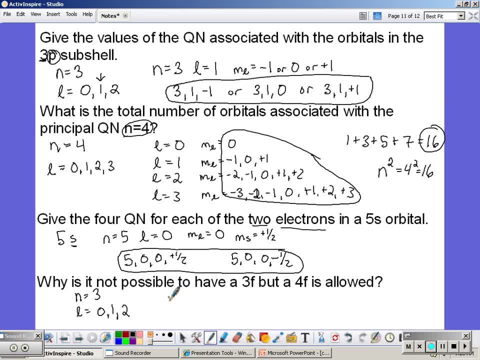 because f would mean L is equal to 3.. Now if N is equal to 4,, our L value can be 0,, 1,, 2, or 3.. So the 4f is allowed because we have L is equal to 3.. 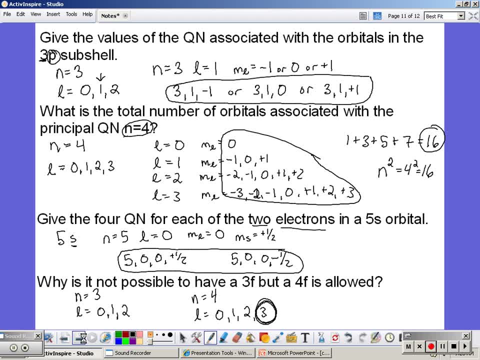 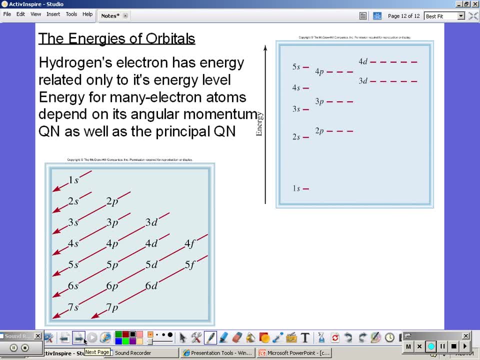 So the energy of the orbitals. Hydrogen's electron has energy related only to its energy levels, But for the many electron atoms it depends also on the angular momentum quantum number As well as the principle quantum number. So we actually get Alphabow's principle And so we fill on the diagonals and there's 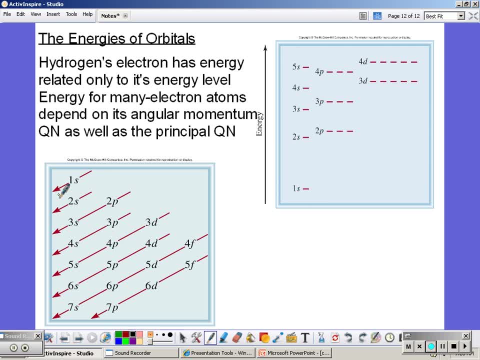 a blip when it comes to the p and the d. So after you fill the 3p, you fill the 4s, then go back and fill the 3d. 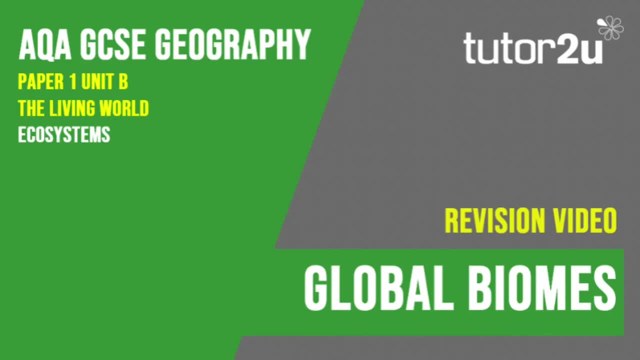 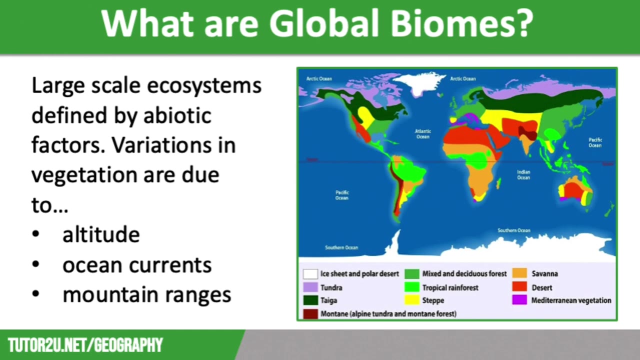 Welcome to this tutor, to you revision video that looks at what global biomes are and runs through the characteristics of the main ones. This is part of paper one, unit B: the living world. We're going to start off by defining what we mean by global biome. A biome is a large-scale.